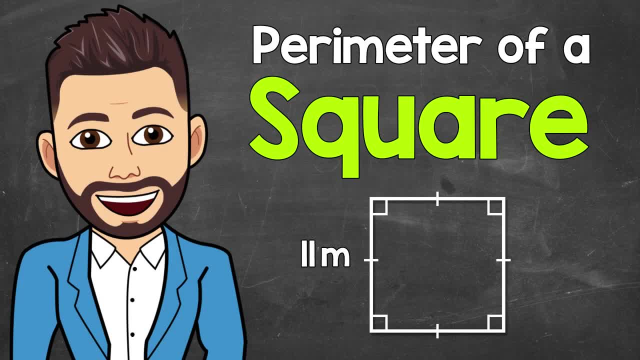 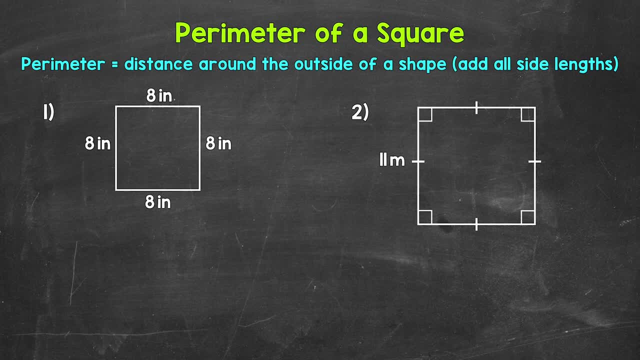 Welcome to Math with Mr J. In this video I'm going to cover how to find the perimeter of a square. Now remember, perimeter is the distance around the outside of a shape. Let's jump into our examples, starting with number one. So let's find the perimeter of this square and we can do. 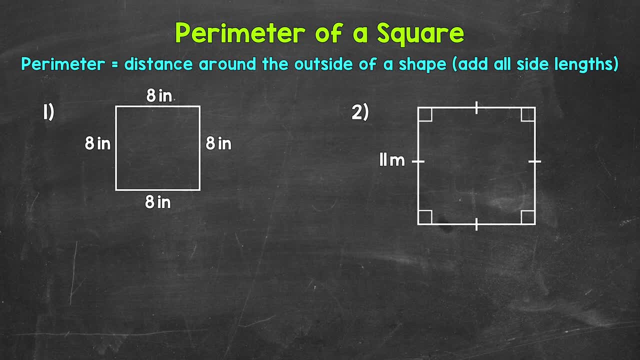 this by adding the lengths of all of the sides. Now for this square, each side is 8 inches, So we have 8 inches, 8 inches, 8 inches and 8 inches. So perimeter equals 8 plus 8 plus 8 plus 8.. 8 plus. 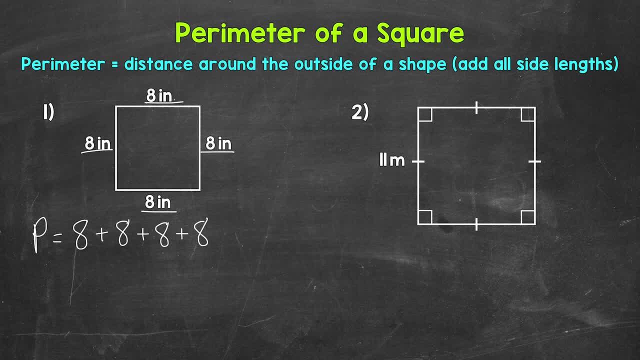 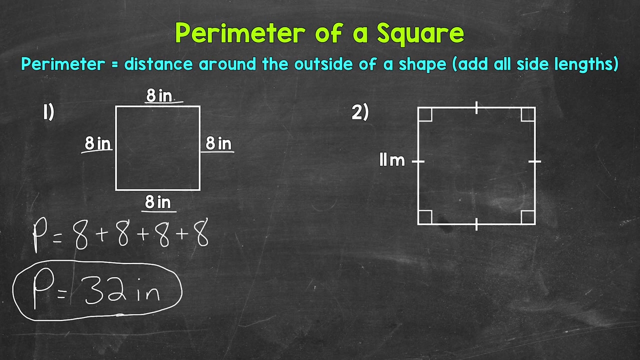 8 is 16, plus 8 is 24, plus 8 is 32.. So the perimeter is 32 inches. That's the distance around the outside of that square. Now I do want to mention: for squares, we can just multiply a side length by 4, since all of the sides are the 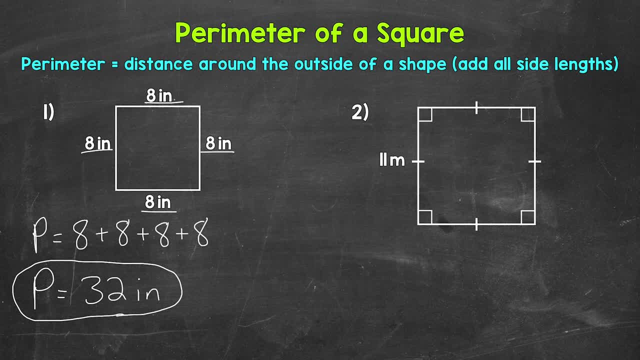 same. Instead of 8 plus 8 plus 8 plus 8, we can just do 8 times 4.. We get the same thing either way. We can use the formula: perimeter equals 4s, 4 times a side length For this square. each side is: 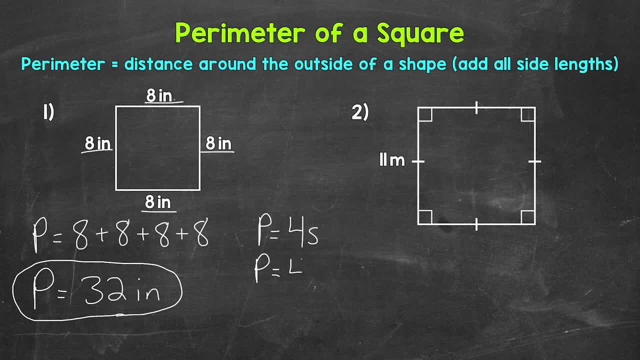 8 inches. So let's plug in 8, 4s, So 4 times 8.. 4 times 8 is 32.. So the perimeter equals 32 inches that way as well. So for the perimeter of a square we can either add all of the 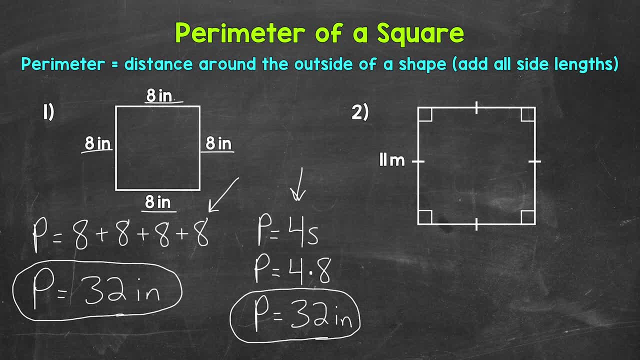 sides, or we can multiply a side length by 4.. Either way will work. Let's move on to number two, where we have a square with sides that are 11 meters, and you'll notice that we only have one side labeled. That's because this is a square and we know all of the sides are. 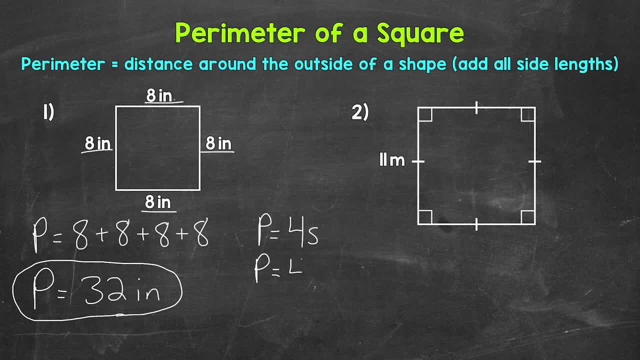 8 inches. So let's plug in 8, 4s, So 4 times 8.. 4 times 8 is 32.. So the perimeter equals 32 inches that way as well. So for the perimeter of a square we can either add all of the 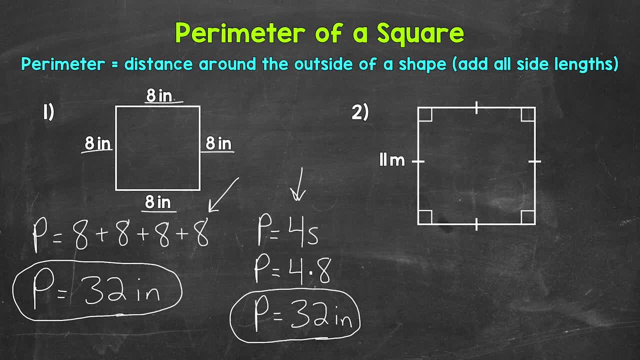 sides, or we can multiply a side length by 4.. Either way will work. Let's move on to number 2, where we have a square with sides that are 11 meters, And you'll notice that we only have 1 side labeled. That's because this is a square and we know all of the sides. 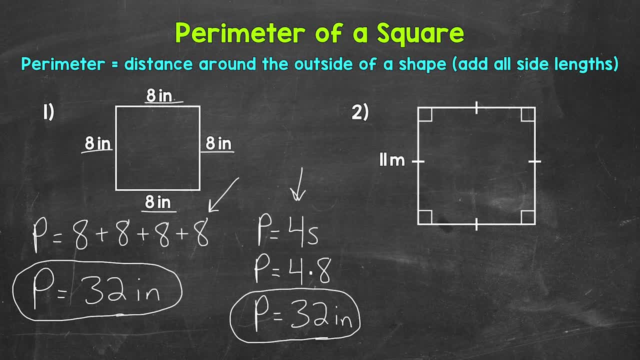 are the same, So all of the sides are 11 meters. These tick marks right here Show us that all of the sides are the same. We have one tick mark on each side indicating that they are all again the same. 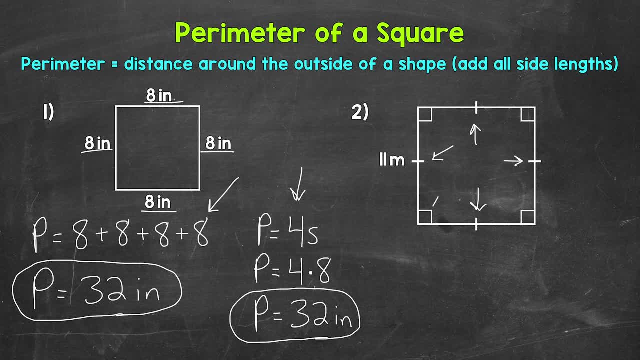 They are all 11 meters. Then we have right angle symbols as well, 90 degree angle symbols. I wanted to include all of these symbols in case you come across them. That way you will know what they mean. So something to keep in mind. 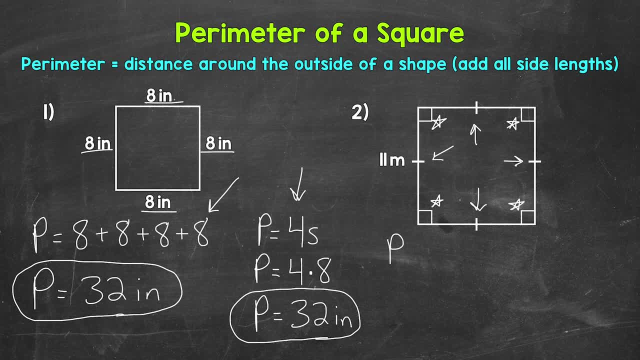 As far as perimeter, let's start by adding all of the sides, So we have perimeter equals. Again, all of the sides are 11 meters. So 11 plus 11 plus 11 plus 11.. 11 plus 11 is 22 plus 11 is 33 plus 11 is 44.. 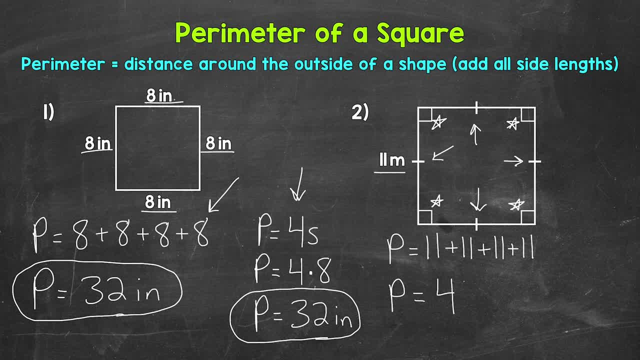 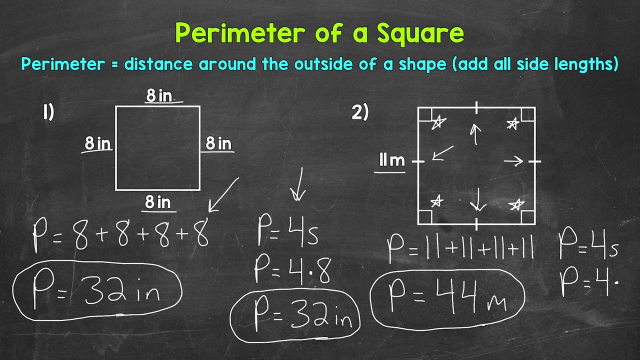 So the perimeter is 44 meters. Now we can also find perimeter of a square by multiplying a side length by 4.. So we can use the formula perimeter equals 4s. Let's plug in 11, 4s, So 4 times 11.. 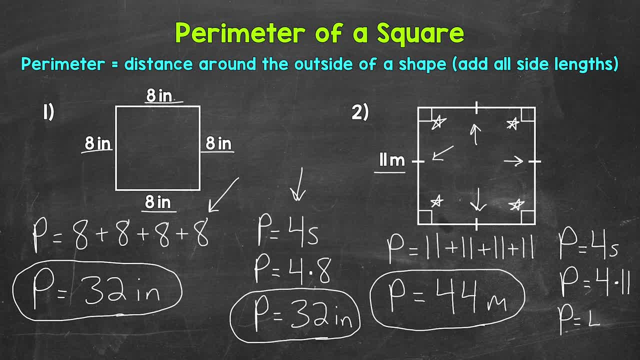 4 times 11 gives us a perimeter of 44 meters That way as well. So again, we can find the perimeter Of a square by either adding all of the side lengths, So all four sides, or we can multiply a side length by 4, since it's a square and all of the sides are the same.